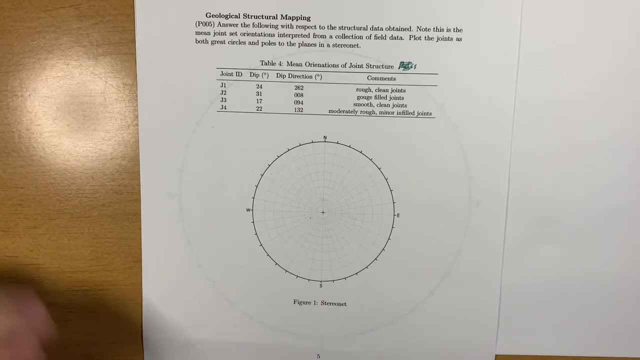 tutorial. So what do we do with these geological structures? Well, we get some sense of sort of the dominant structures that occur in certain tunnel conditions. Oftentimes we do some kind of statistical analysis to look at the joint sets and so on, And it's really important to understand, to give you some way of assessing whether wedges and so on are like. 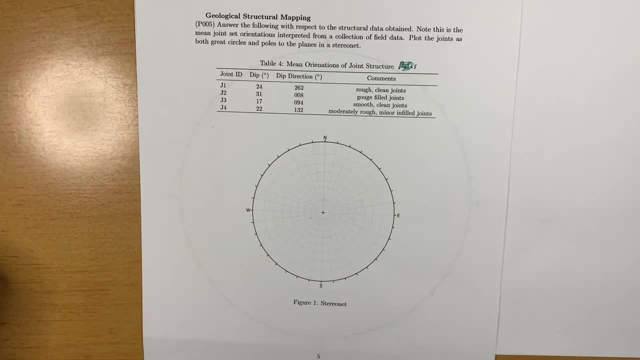 basically to form around your excavation what their dimensions are, how they're going to intersect the excavation, which may be at different orientations, And really to aid us in doing sort of a limit equilibrium of a wedge and its stability. Okay, so the question is to basically to plot the joint set information on a stereo net. 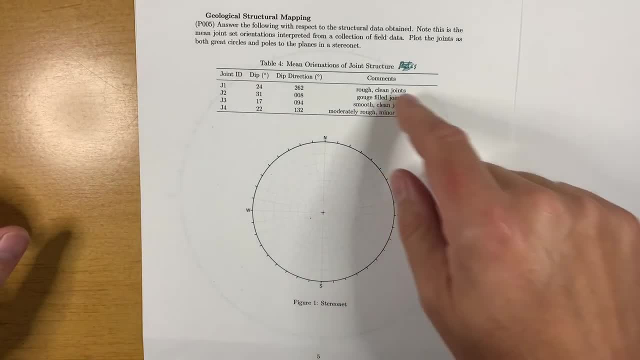 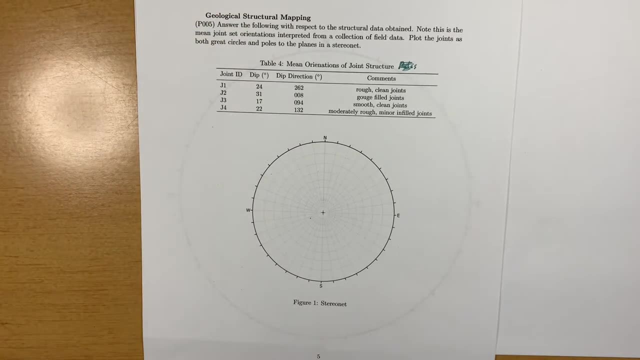 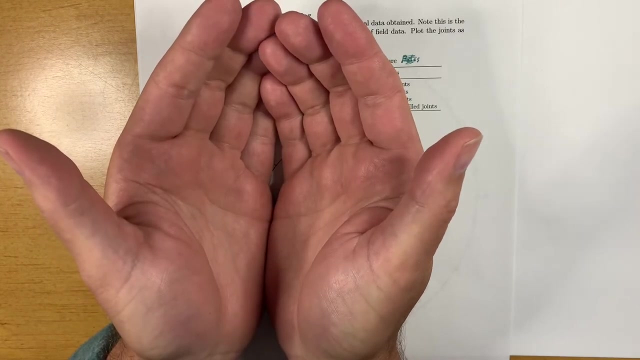 We're given dip and dip direction of the joint sets and a little bit of information about it. It's also asking us to plot the plane, the pole to the plane. So we're going to plot both of the plane and the pole to the plane. So if you recall briefly, basically the stereo net is a way of visualizing a lower hemisphere of a sphere. 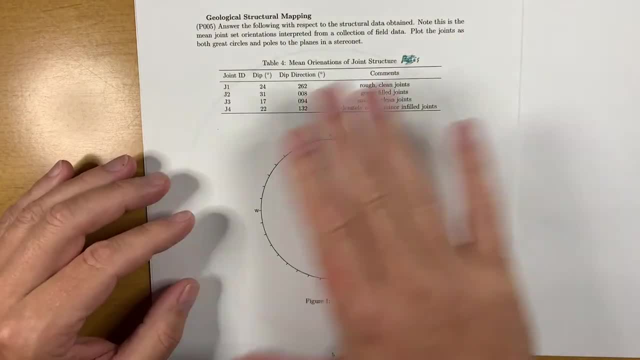 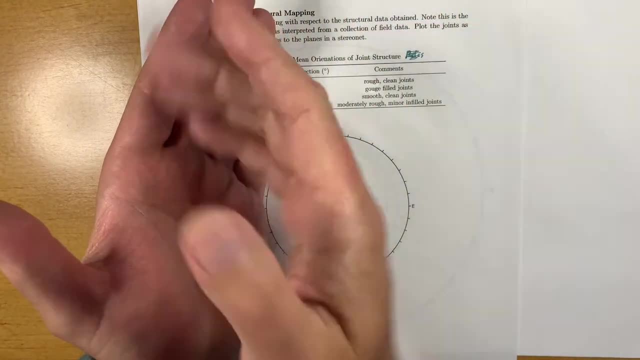 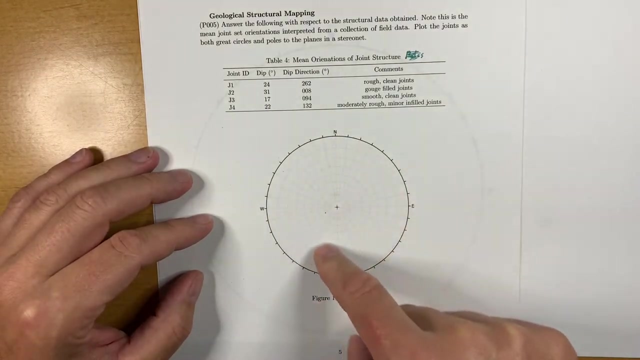 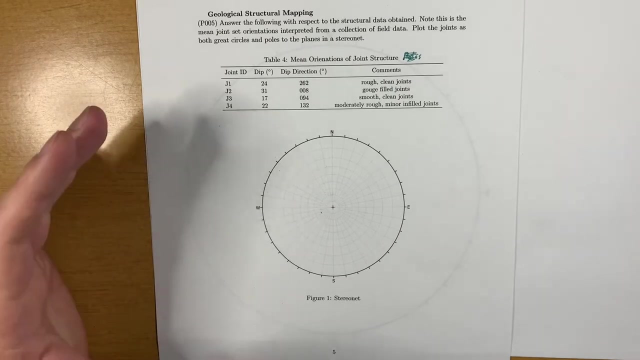 In two dimensions and essentially the planes intersect the bottom of the lower hemisphere, And in 2D they are projected as a great circle, Okay, so sort of a half moon arc type circle, depending on the dip and dip direction And the pole of the plane is the normal to the plane. 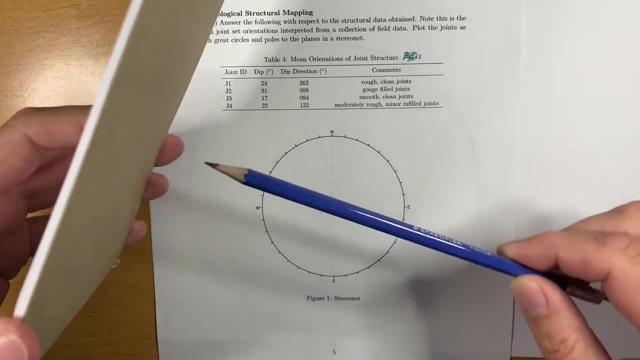 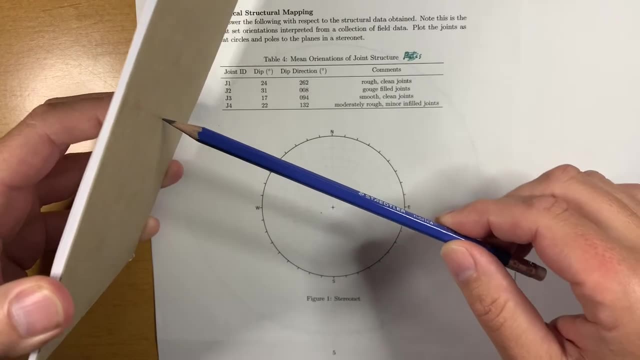 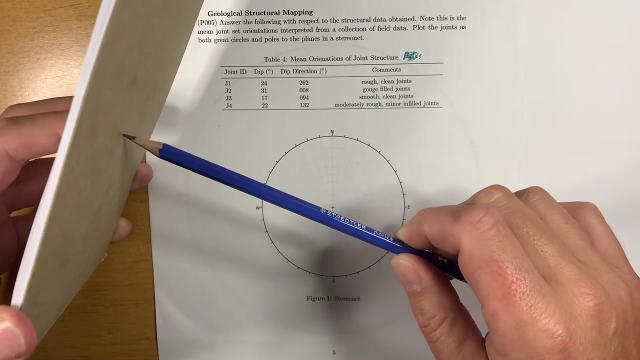 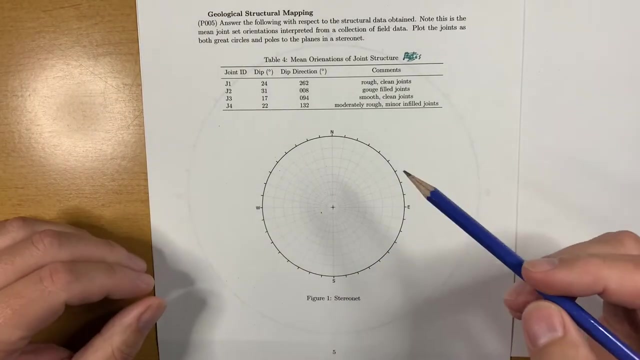 Okay, so we have a great circle for the plane itself And then, for example, the pencil would be sort of the normal if, if the pad here was the plane right and it's in the normal direction, And where that normal intersects the bottom of the lower hemisphere projection, we have a point, And that point is known as the pole. So if we have a, say, great circle, 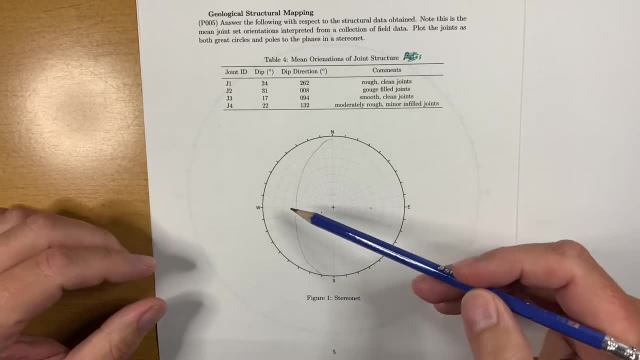 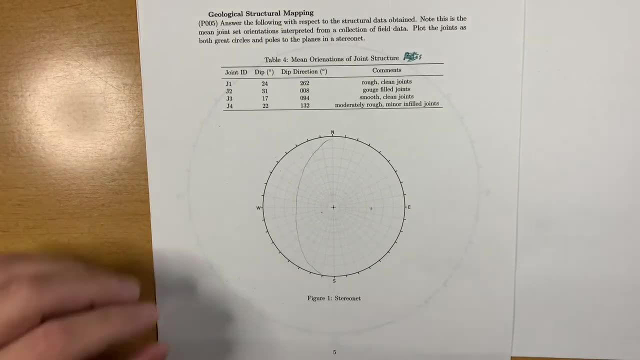 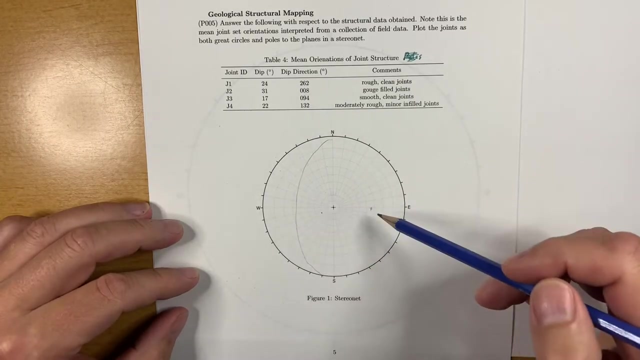 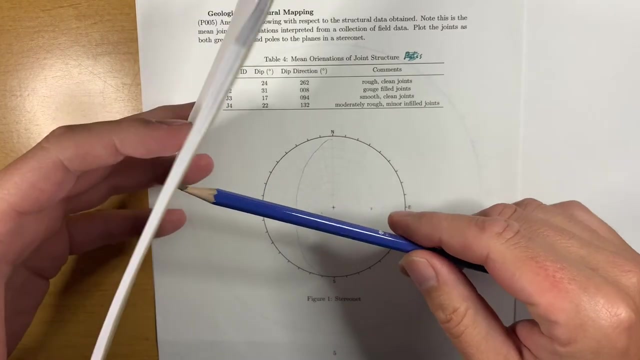 The pole is somewhere over here, right? The, the pole's direction is 180 degrees from the direction of the plane itself. Okay, so that's an easy thing to calculate. And the, the dip. well, first off, the plane and the pole intersect at 90 degrees. right, when we're talking about the dip. 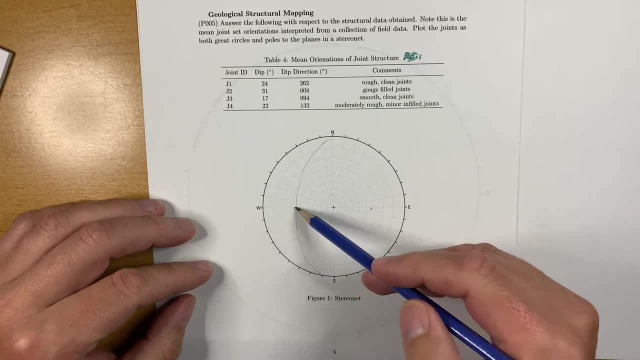 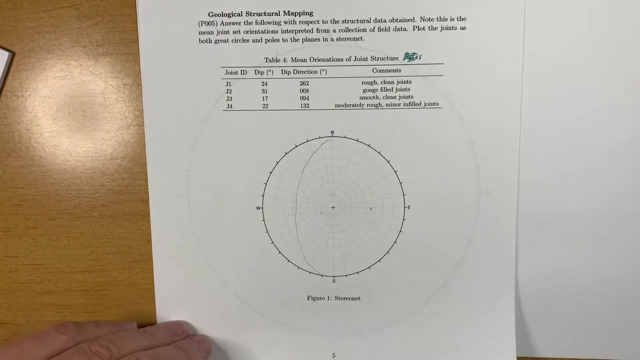 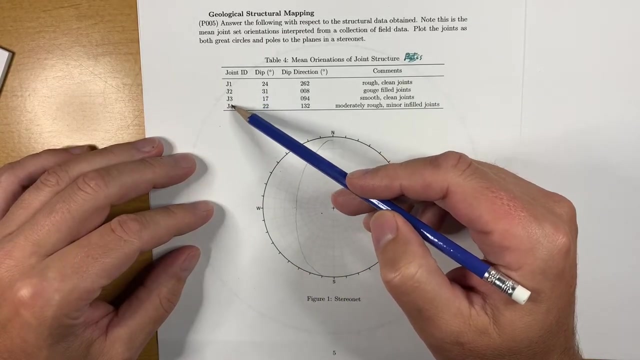 So the dip of the plane Um plus the dip of the pole add up to be 90 degrees. Okay, so we'll we'll explain that a bit more when I give you some examples. What do we have here? We have four joint sets: J1,, 2,, 3, and 4. We have some dip angles. Okay, so that's the dip below the horizon. 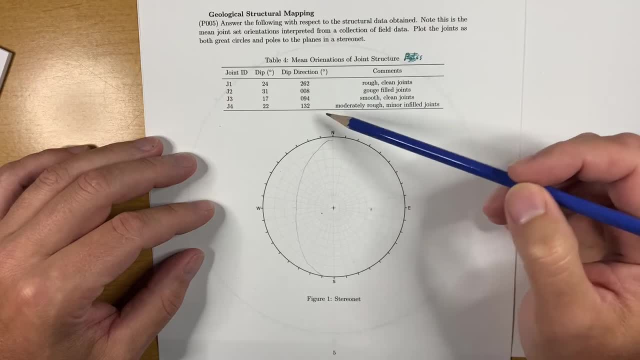 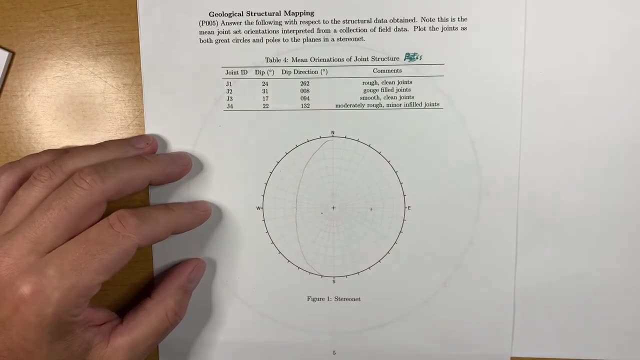 And we have some dip directions which are compass angles, and they're always reported with three digits Um, so that really you don't get them confused with the dip. And then we have some comments here about it: Rough, clean joints, right. 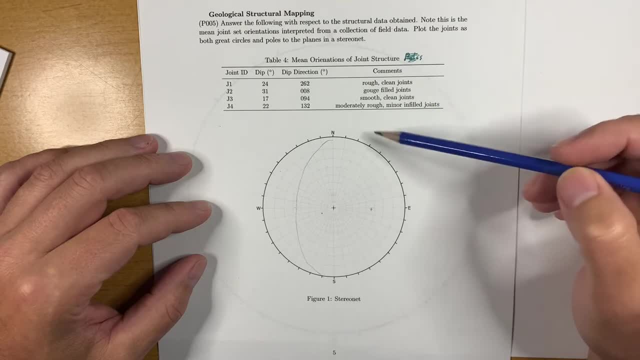 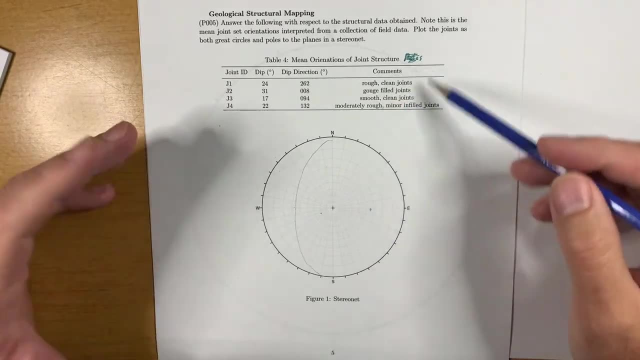 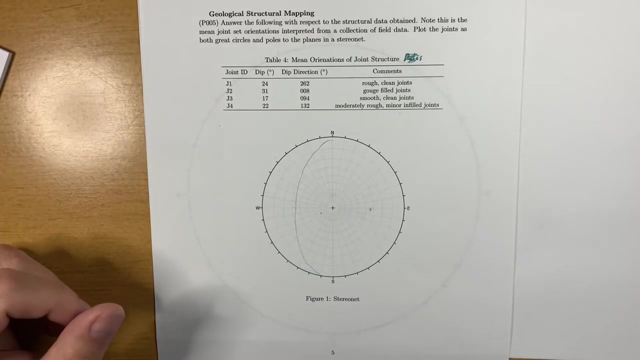 Gouge filled joints. smooth, clear, clean joints, moderately rough, with minor infill joints, Okay. but uh, you know you could have other structures as well. You could have faults um schistosity, um bedding planes. you know those kinds of things could also be included. 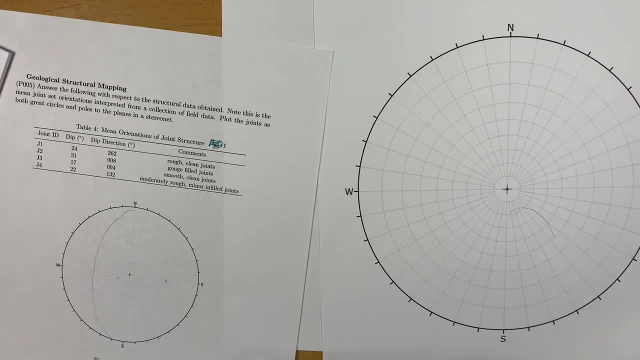 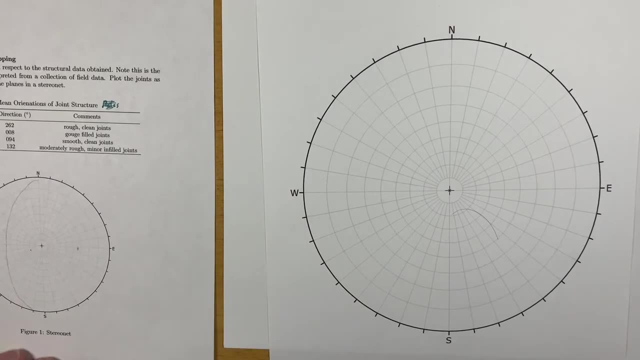 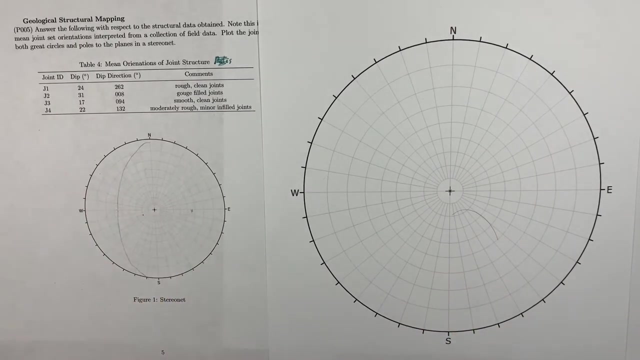 Okay, I have here a blown up version of that stereonet And we're gonna use that to plot these structures. I'll try to do it so that we can sort of see both at the same time. Okay, So first off. 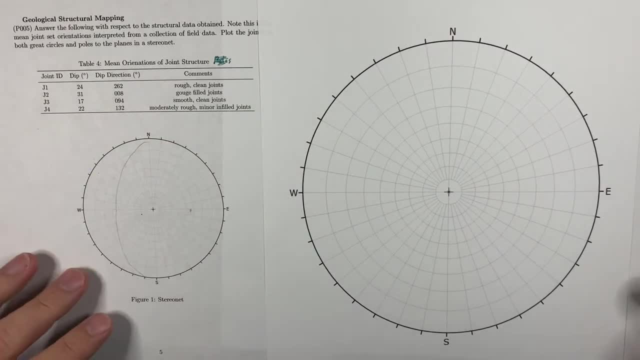 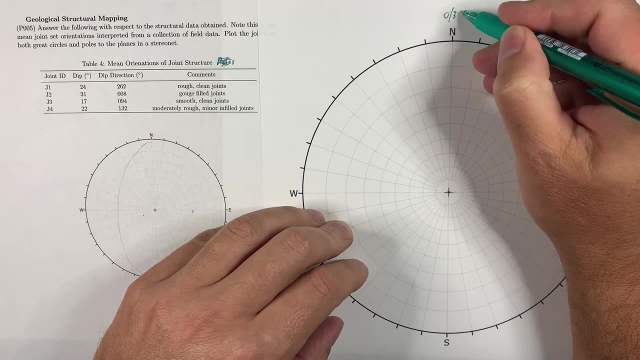 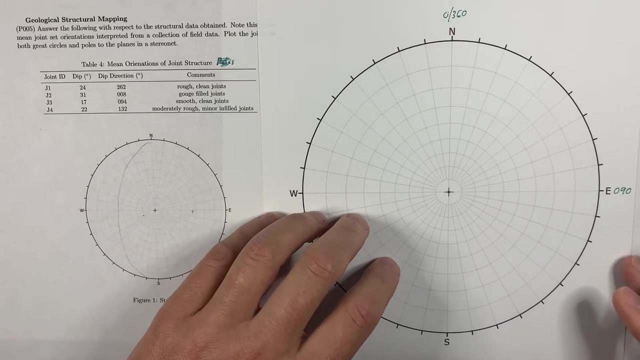 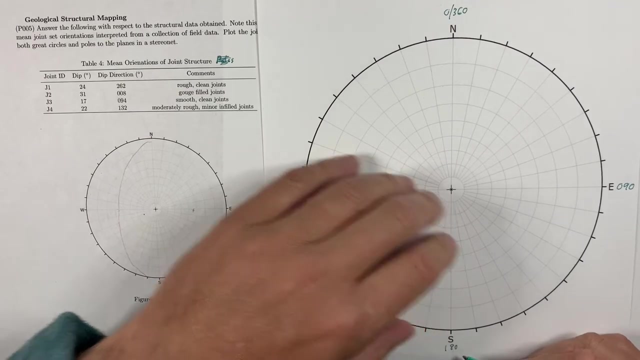 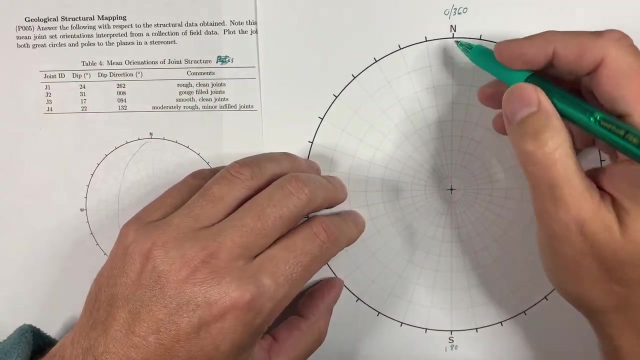 we have our stereonet here and let's draw in. So we got zero and 360 degrees is north, and then we have 90 degrees is east and then south. we have 180 degrees west, 270 degrees and the dip below the horizon, you know, for something in the north is. so it's zero. 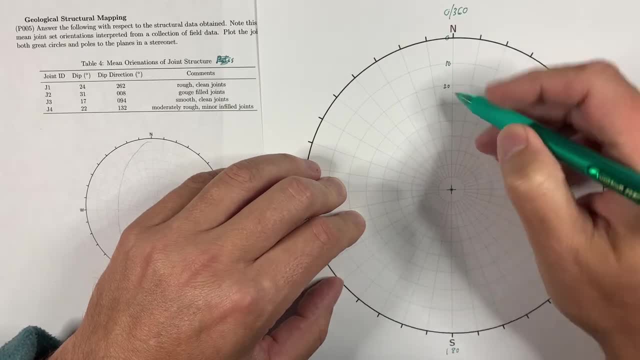 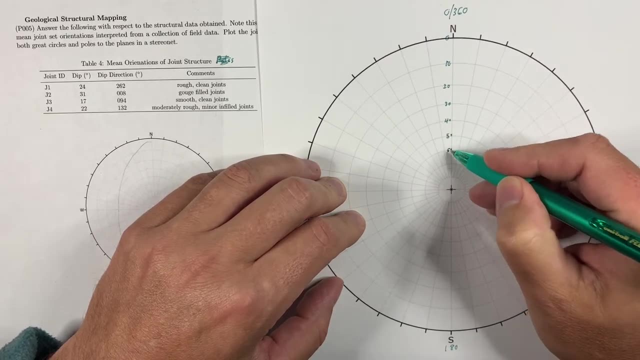 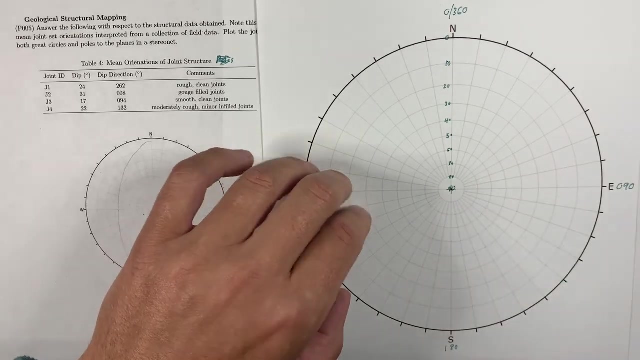 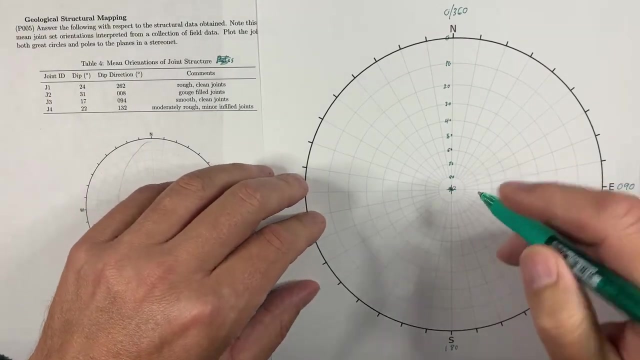 10,, 20,, 30,, 40,, 50,, 60,, 70,, 80, and 90, or vertical, okay. So something will plot on the rim if it's horizontal, like a horizontal bedding plane, and it will plot in the middle if it's exactly vertical. okay. 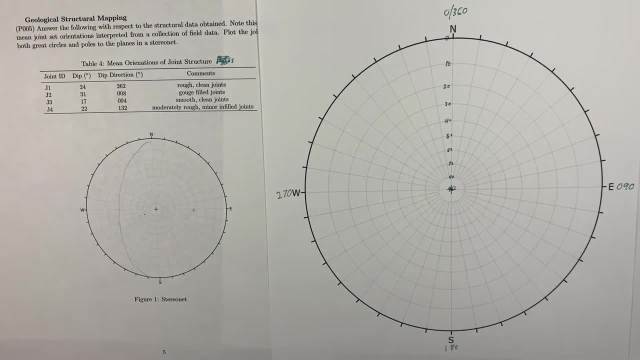 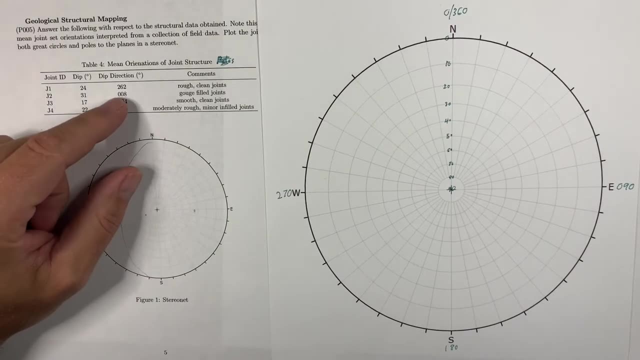 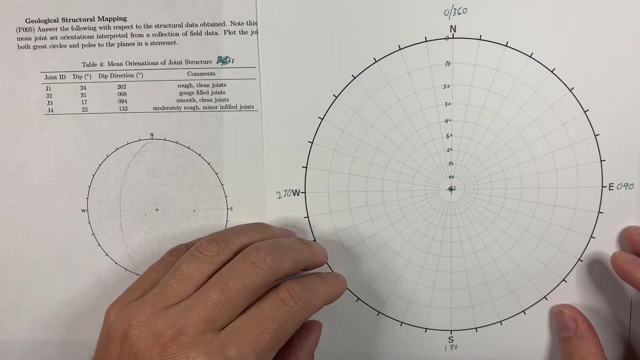 All right. So let's look at our structures that we want to plot here. So the first one has a. let's try and establish the dip direction first before we look at the dip. So we are talking about a dip direction of 262.. 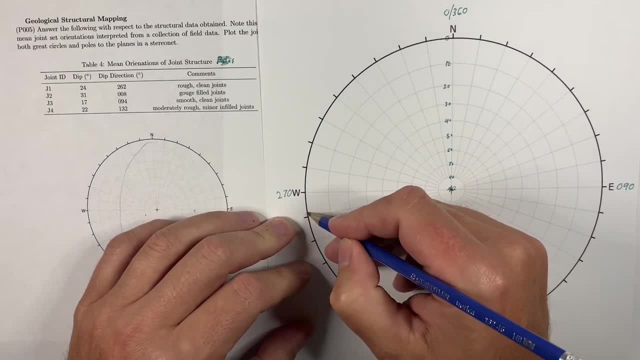 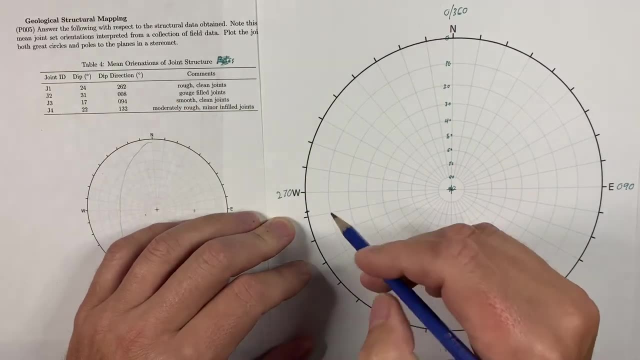 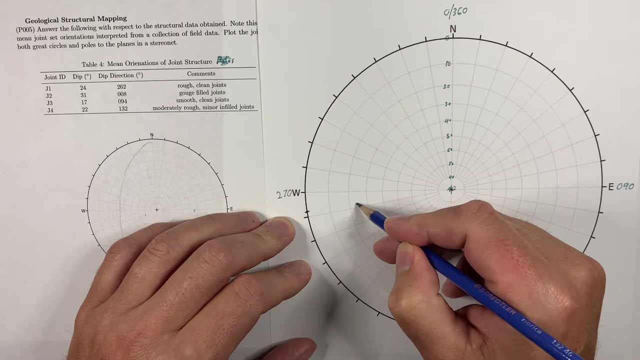 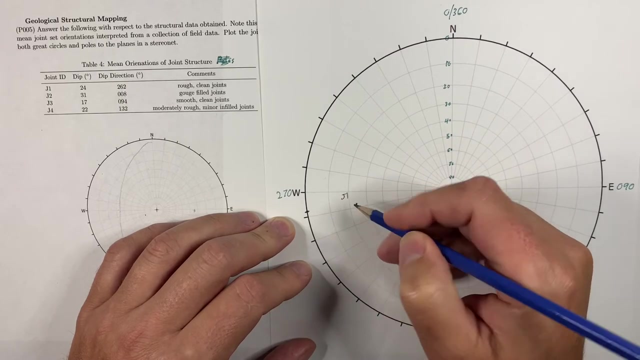 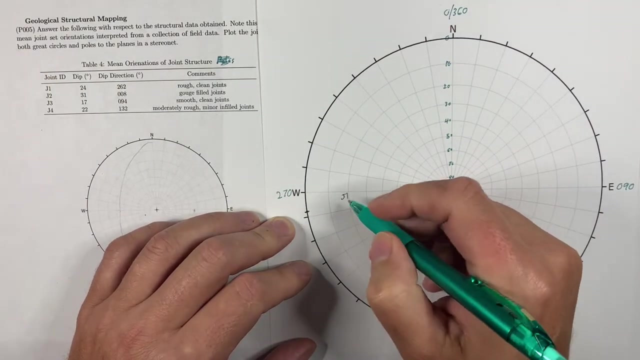 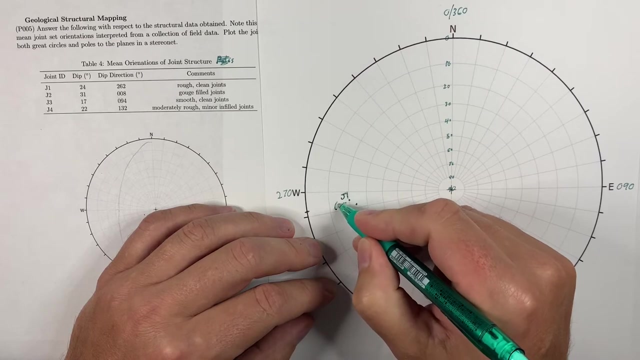 So 262,, okay, And the dip is 24.. Okay, so we're dipping 10,, 20,, 25 is the middle, 24, okay, right there, right. So that is J1, and its dip is actually- I'll do this in pen, make it a little nicer for you- J1,. so we'll plot it with dip of 24,. 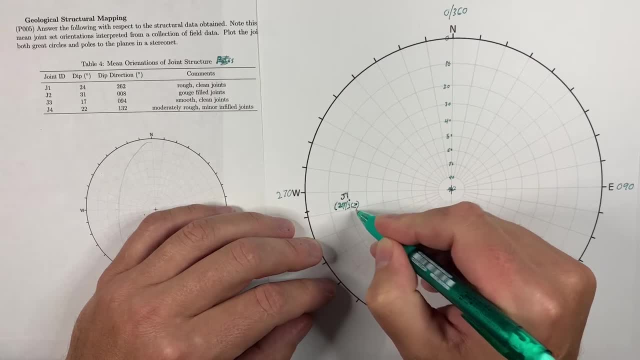 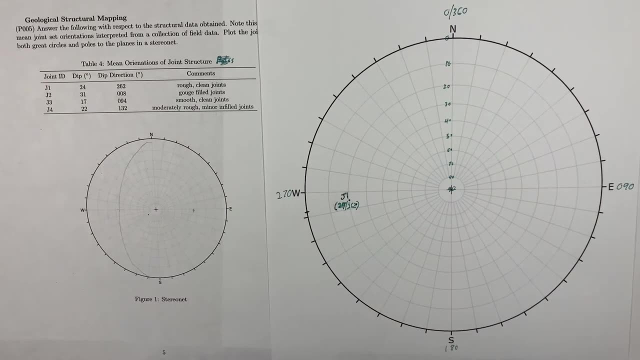 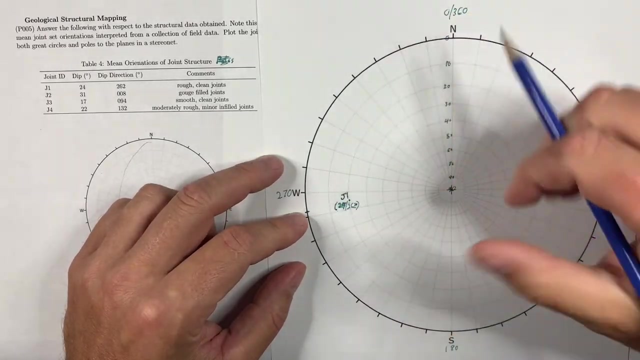 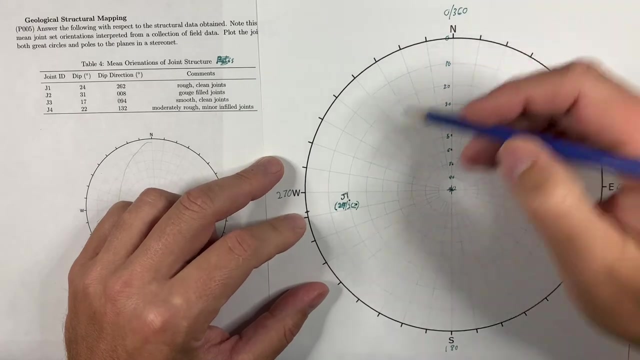 262 is the dip direction. okay, A little bit hard to see there, okay. So now we want to plot the great circle, So we want to go and tick off two points at 90 degrees to have where the ends of the great circles intersect- the outside- okay. 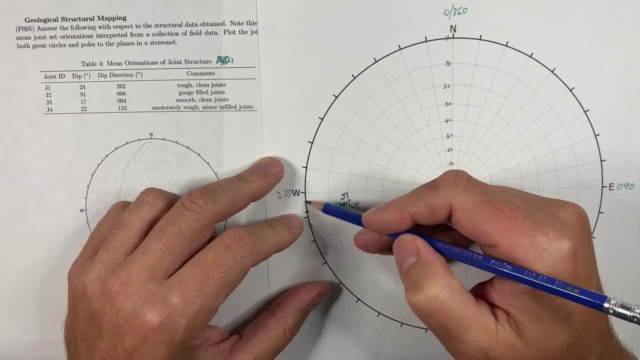 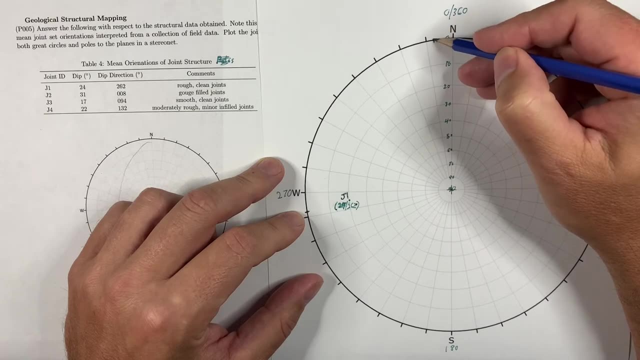 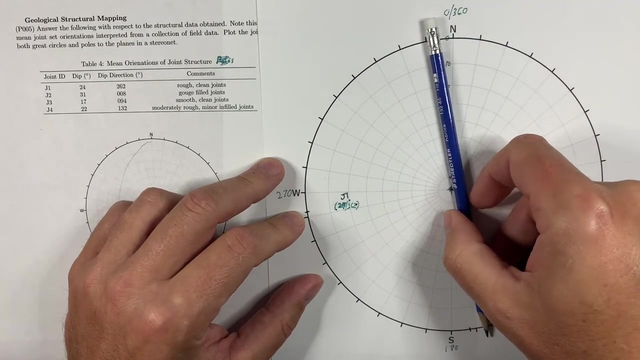 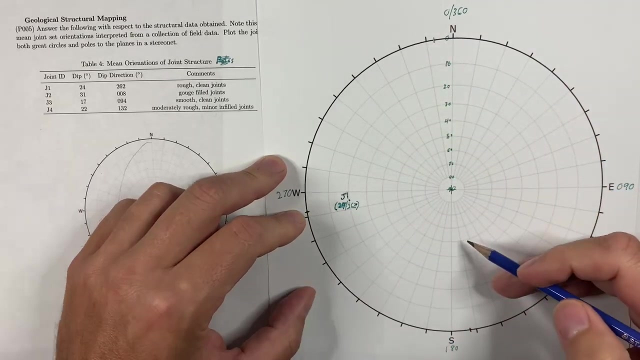 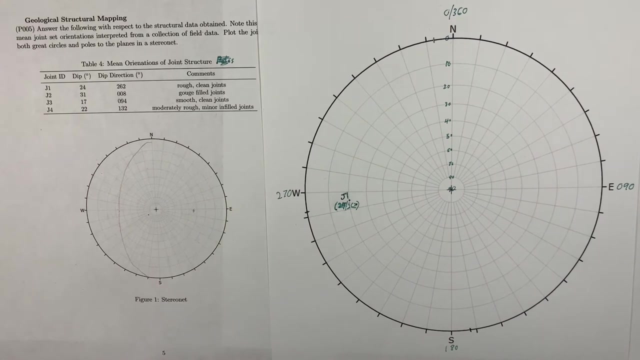 So we're eight degrees. Okay. So we're going to go eight degrees from west, So we can just go eight degrees from north and approximately eight degrees from the south. okay, So that is essentially 90 degrees And your great circle is going to go through these two points and right through the apex described by the dip and dip direction and make a nice smooth, clean circle. 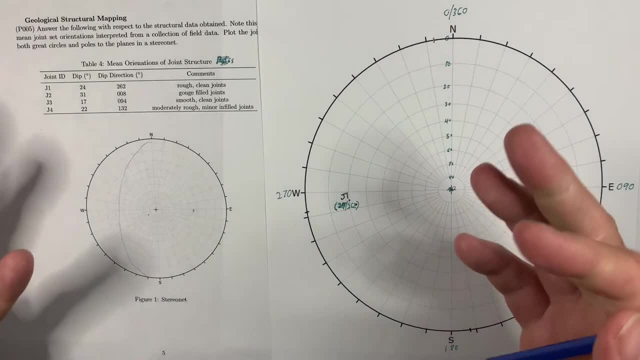 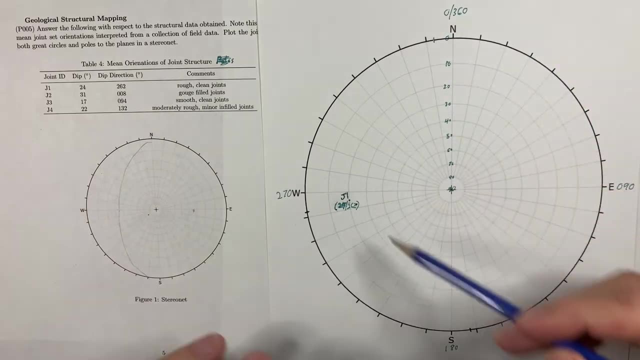 Now there are techniques where you can do that. There are techniques where you can use onion paper or tracing paper and you can use a nice stereographic projection and rotate these and draw these beautiful great circles, And really I probably should be teaching you how to do that. but the reality is we are going to be using the computer for all of this stuff and essentially I just want you to understand how they work and what the numbers are. 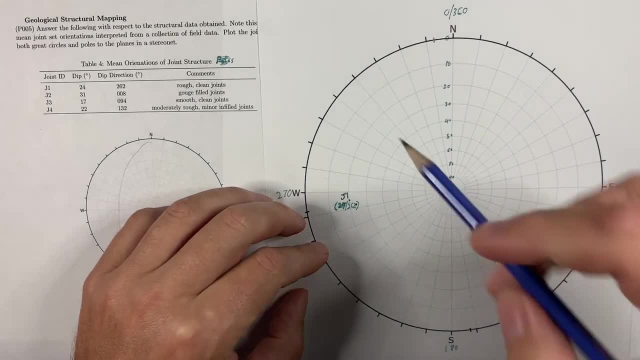 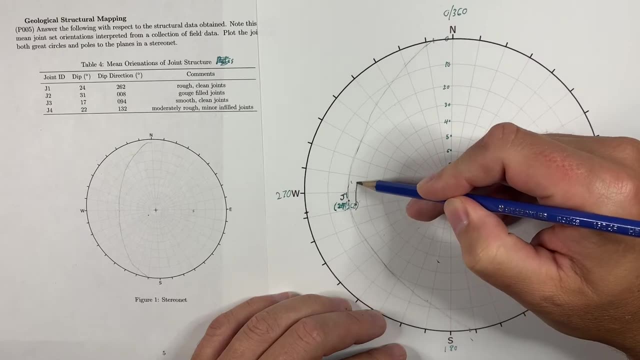 But just to give you guys a little bit of an idea, you can just go in here and draw a circle. I'm not going to do that step of drawing the beautiful great circles, I'm instead simply going to crudely sketch it here. 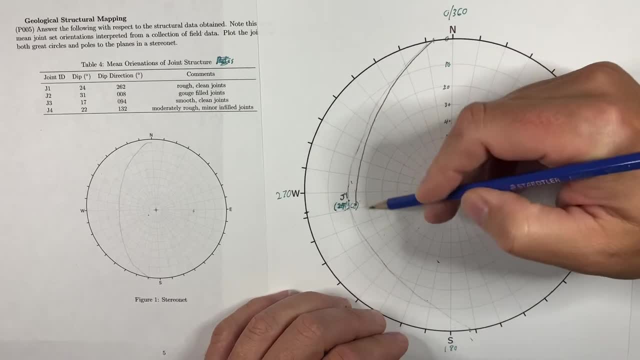 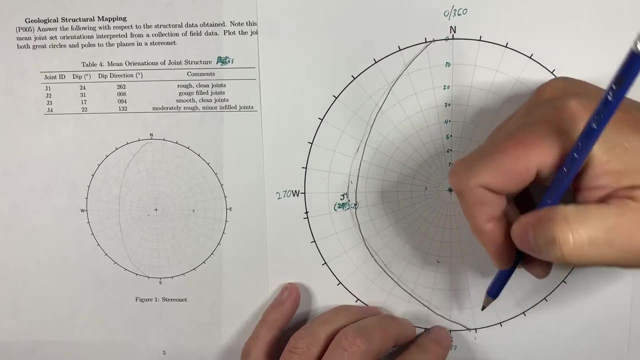 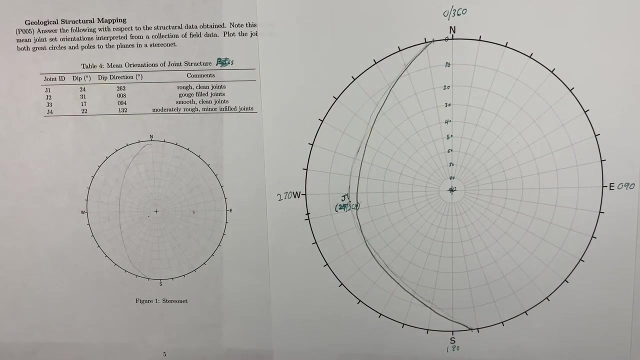 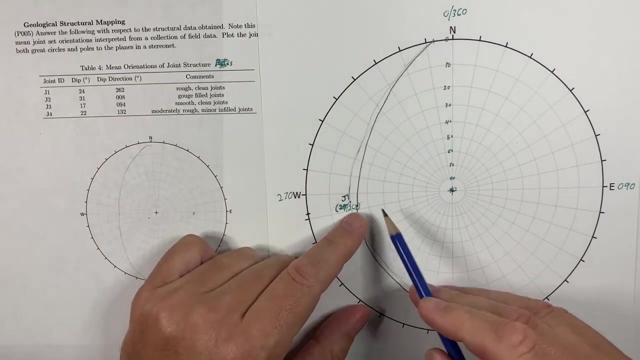 I'll just show you these three. Okay, Okay, I'll just show you this. All right, Okay, Okay. so that is the great circle there, crudely drawn. Now I'll just go ahead and plot the pole. Okay, so the direction of the pole is 180 degrees from the direction of the apex of the great circle, right? 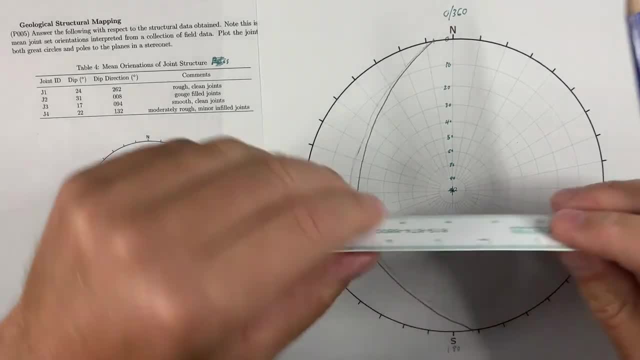 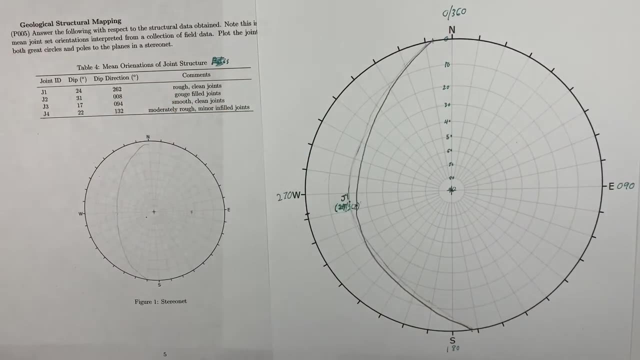 So I could calculate that, or I could simply use a ruler going through the apex and the center and get the direction And for the angle I could either. you know again, they are 90 degrees. The pole and the plane are 90 degrees apart. 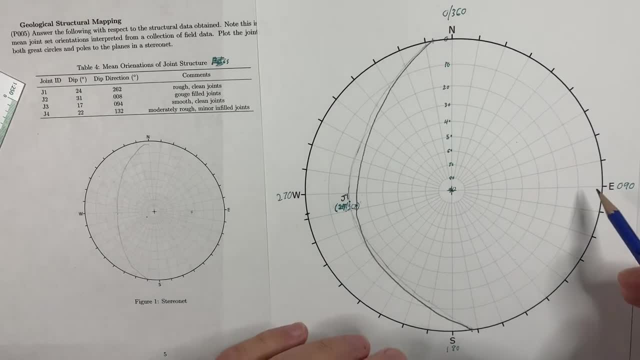 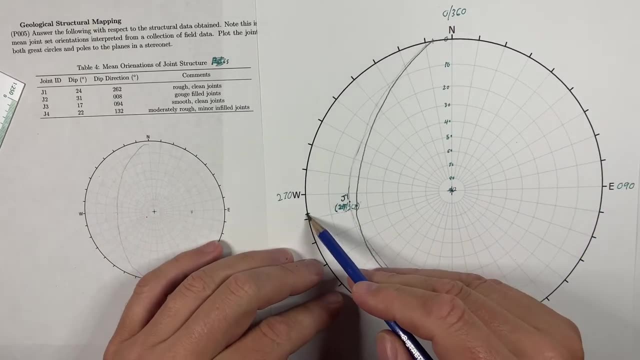 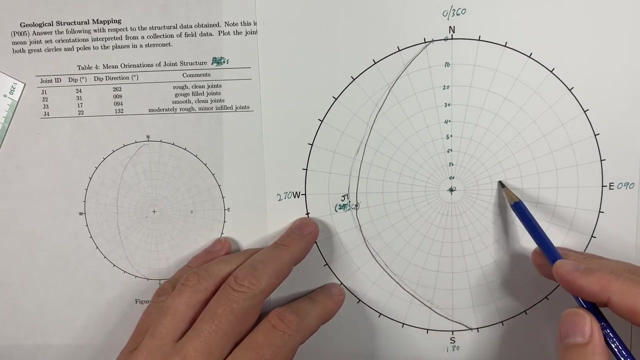 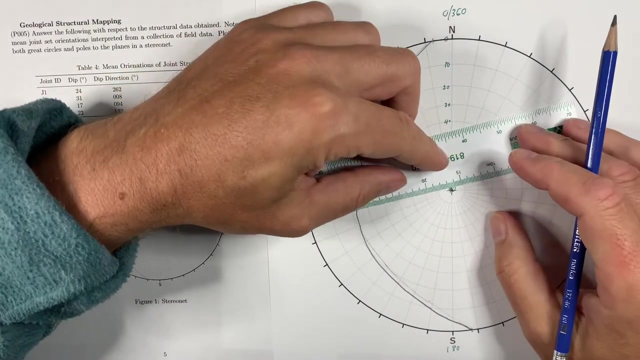 Make a 90 degree angle And I could simply subtract 90 from this and get the other distance. Or, instead of counting down, I could count up the same dip amount and that will be a 90 degrees difference. So this one is 24 degrees right for J1.. 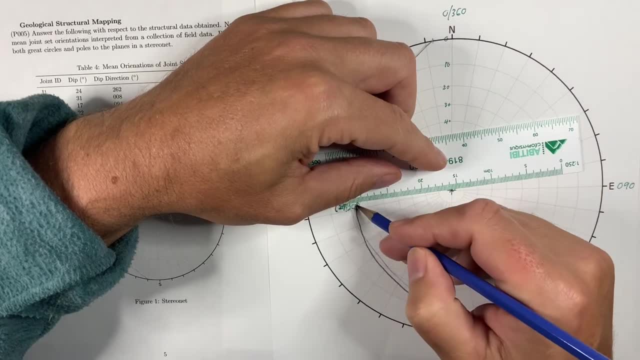 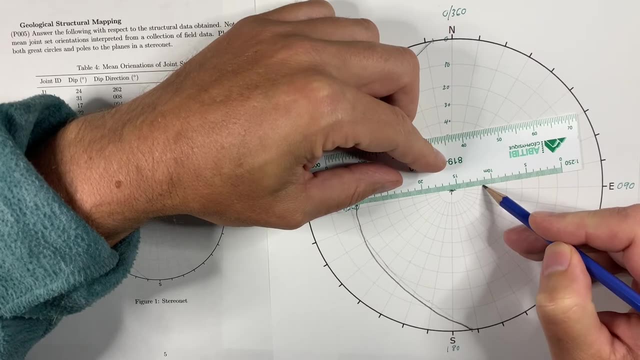 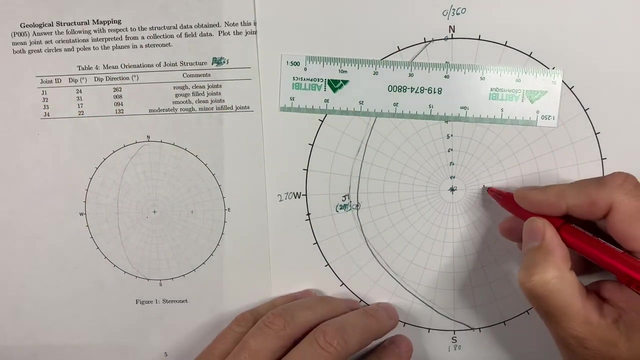 Okay, so I can make sure I pass through the apex point and through the center And 10, 24,. okay is about There. Okay, so I will use a different color here: red for the J1 pole. 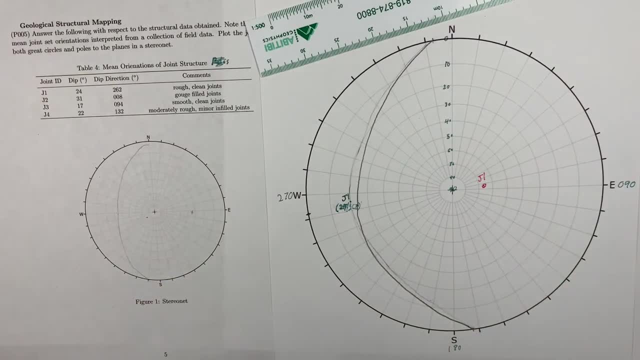 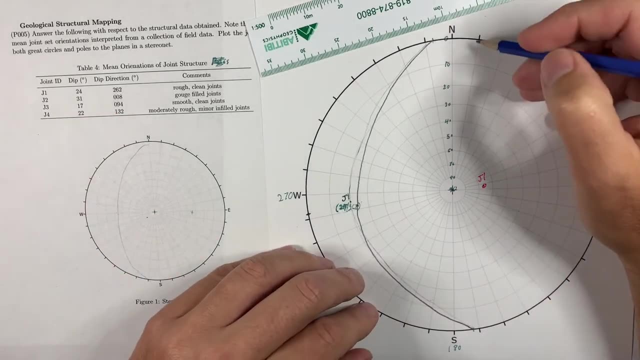 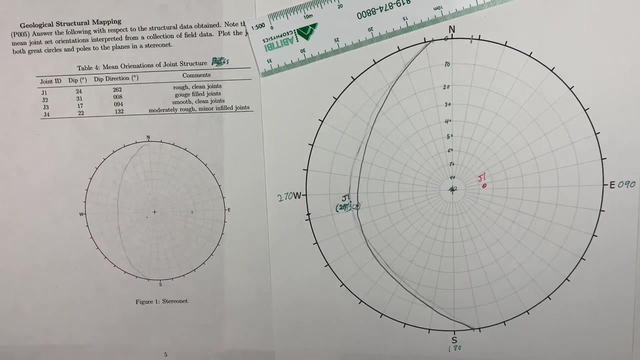 So we have our great circle and we have our pole. Okay, let's do the same thing for J2.. It's 8 degrees, okay, Okay, Right, And it has a dip of 31.. 10,, 20,, 31.. 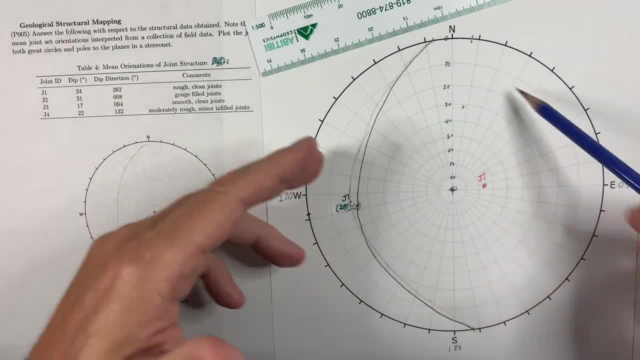 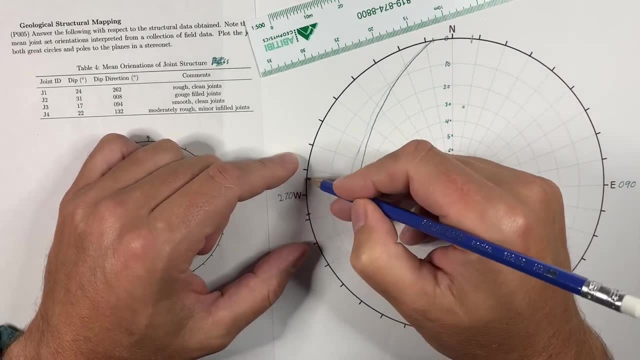 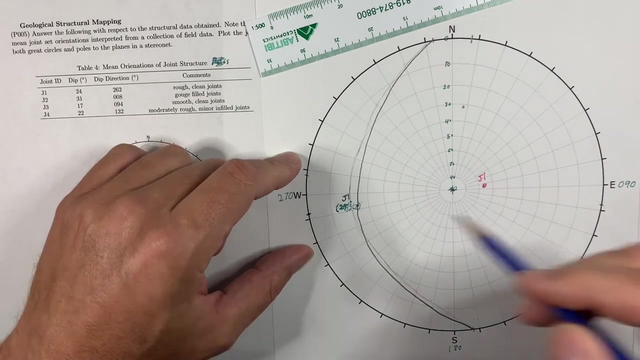 Okay, So now we want to find where the great circle is going to intersect at the outside. So it's 8 degrees from north, We can go 8 degrees from west And we can go 8 degrees from east. Okay, And we need to draw. 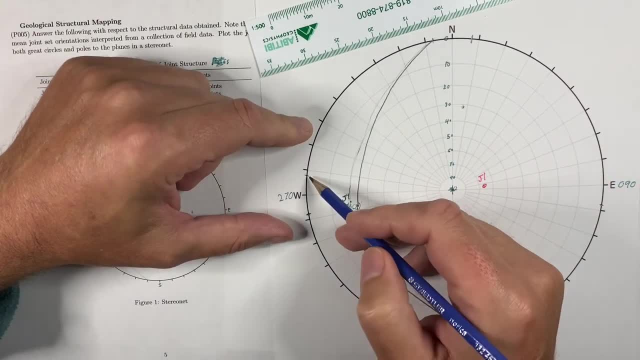 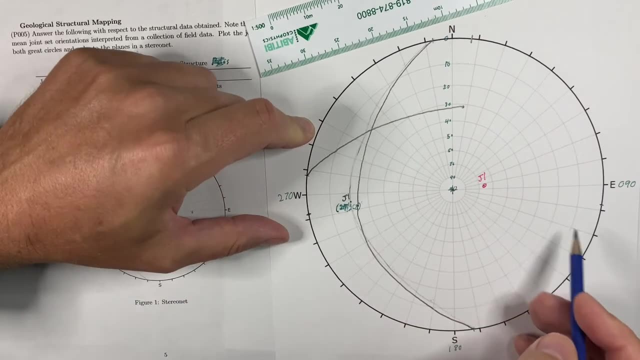 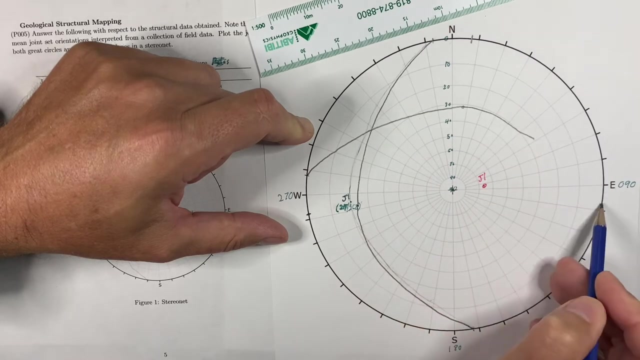 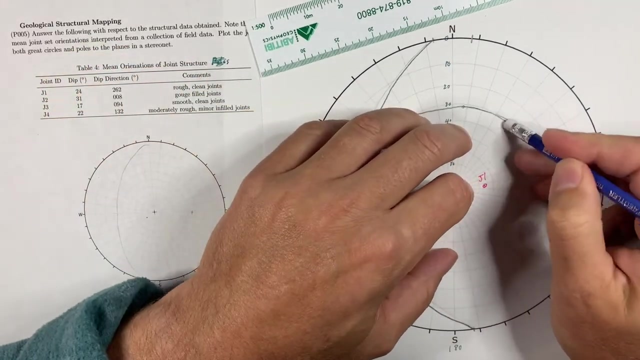 We need to draw a great circle through that point there. Okay, So again, the computer does a much better job. But the computer does a much better job. but let's see what we can do here. Okay, that is not too bad. 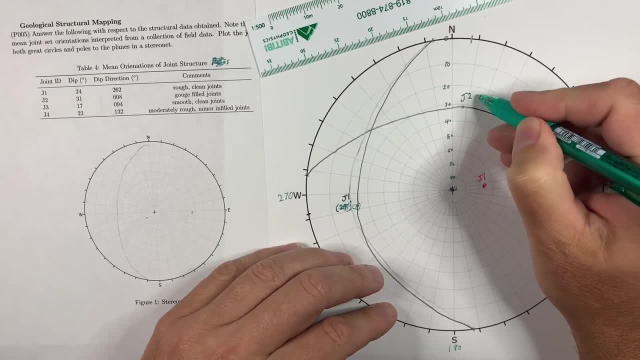 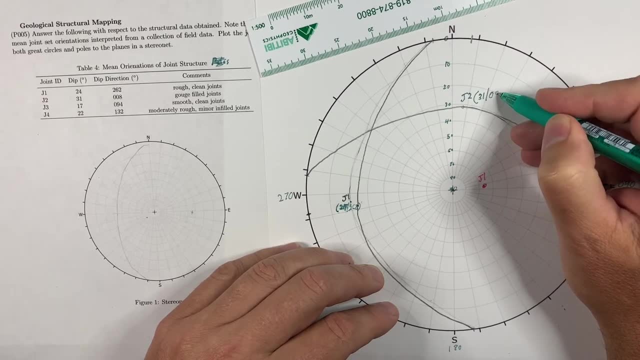 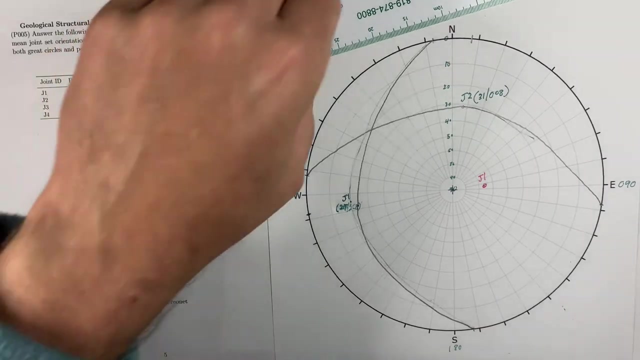 So we will say that's J2, and it has a dip of 31 at a dip direction of 008.. Okay, And you can see how the three digits comes in handy there. Now we'll draw the pole of that one. 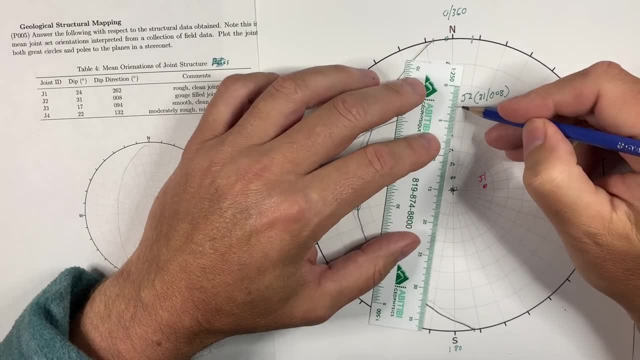 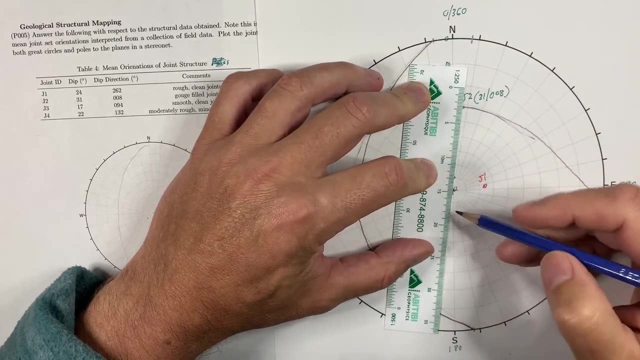 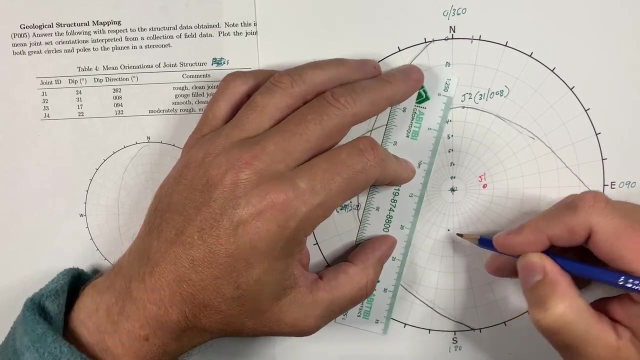 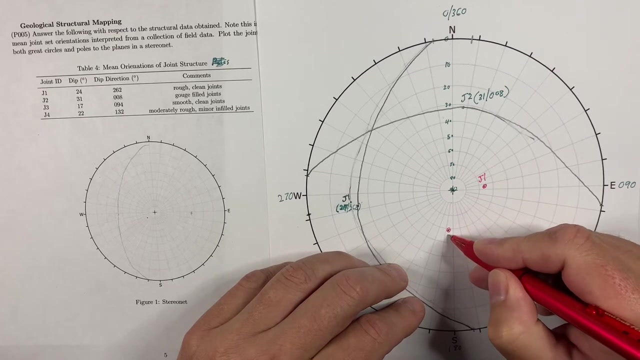 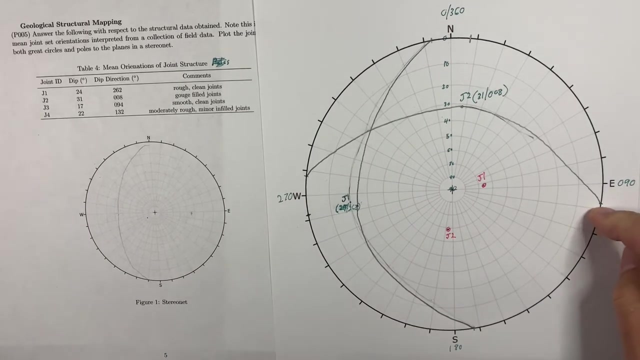 Okay, So we will simply line it up, pass through the middle, and what are we saying? 31.. 31, up this time, 10, 20,, 31 degrees. okay, right there. And that is the pole of J2,. okay, J2,, all right. 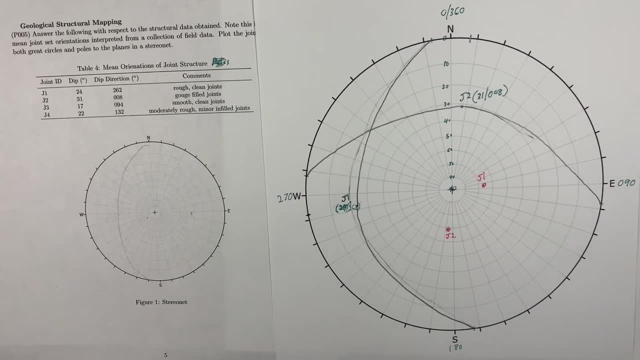 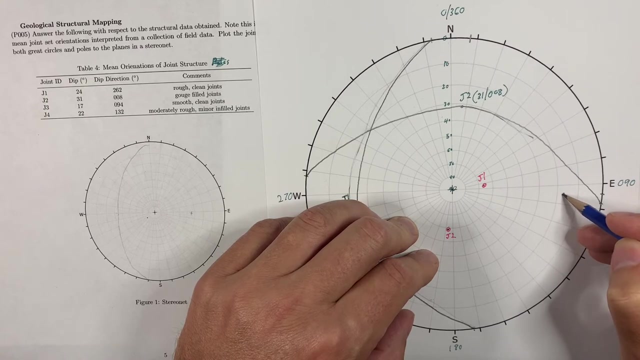 So let's do J3. It's 94 degrees Divided, That's a dip direction 94. And a dip of 17 degrees. 10,, 15, 17 is about here. Okay, And again, let's draw where it's going to intersect at the outside. 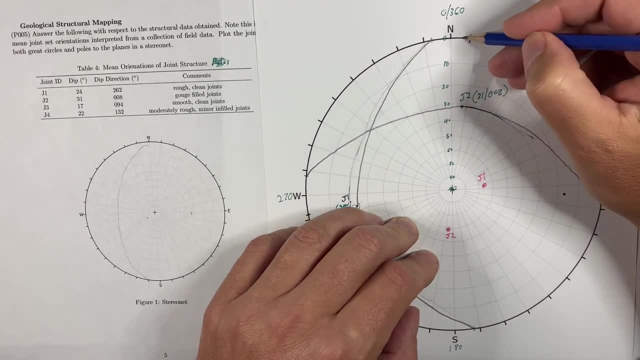 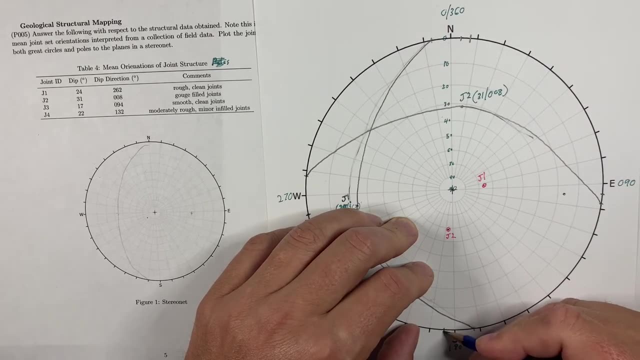 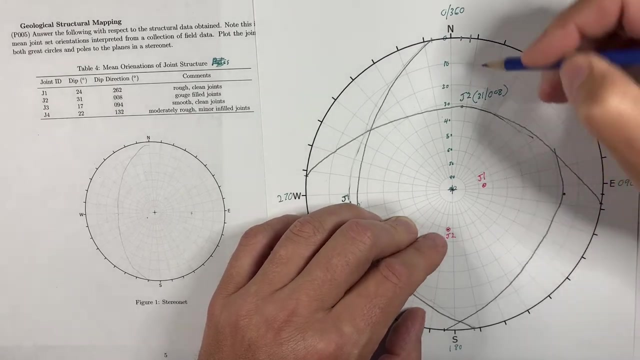 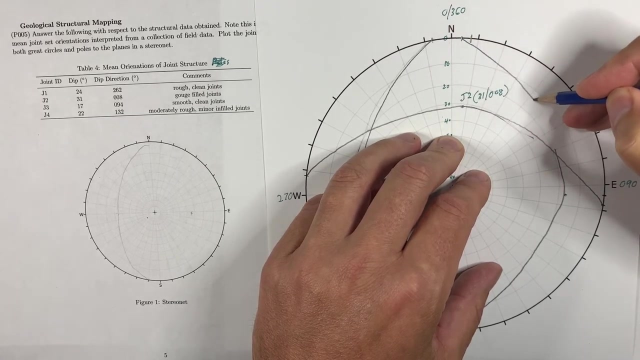 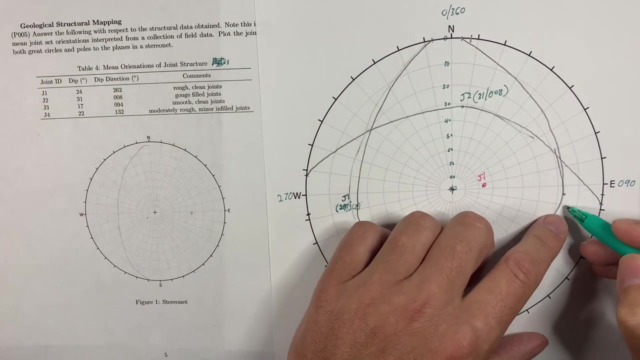 So we want to go 4 degrees past north And we want to go 4 degrees from here. Okay, Cool, to go four degrees past south and draw an intersection here, Okay. so let's label that one. Okay, that is J3 and that is 17 degree dip. 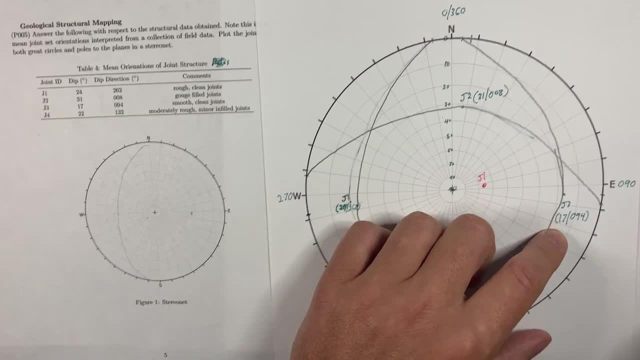 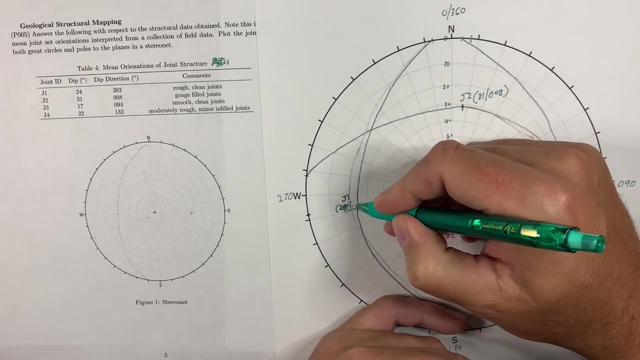 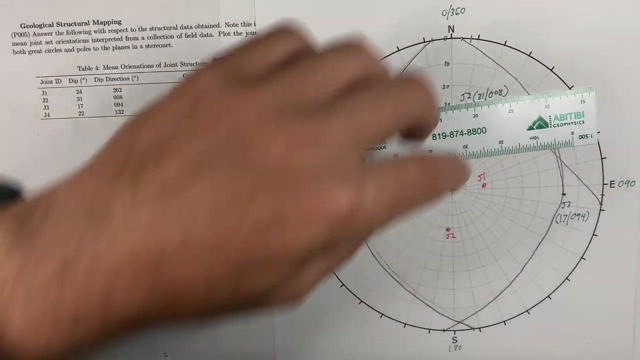 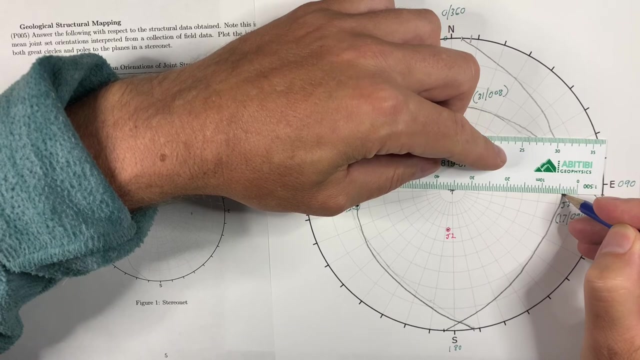 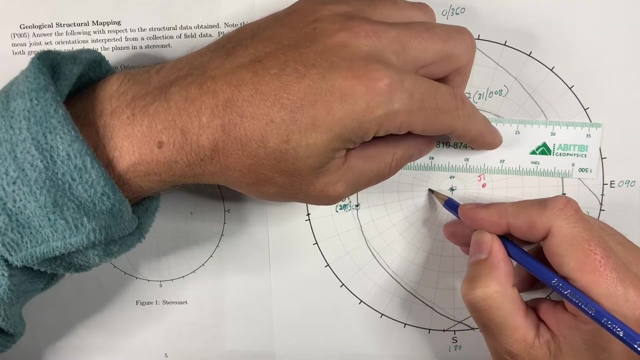 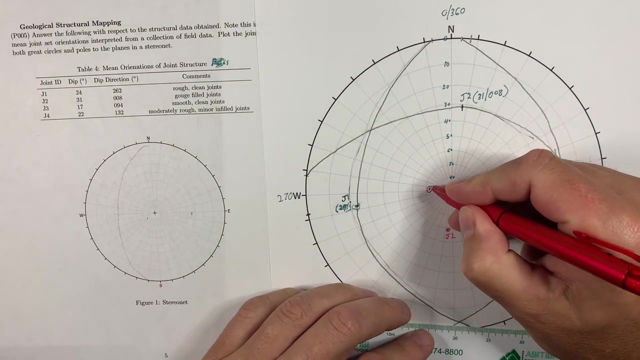 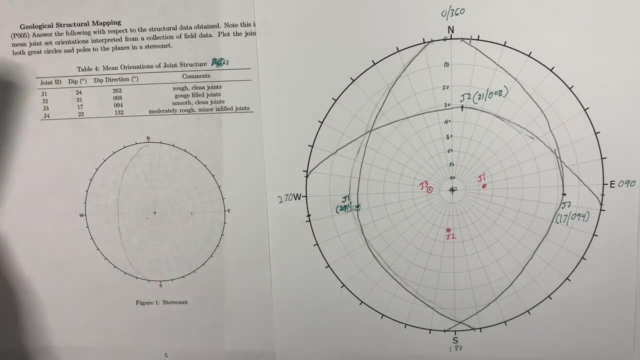 94 degree dip direction. okay, And let's put the pole in here. So let's go through the center and this time we're going to go 17 degrees up: 10,, 15,, 17,, okay. So right here we have the pole of J3, okay. 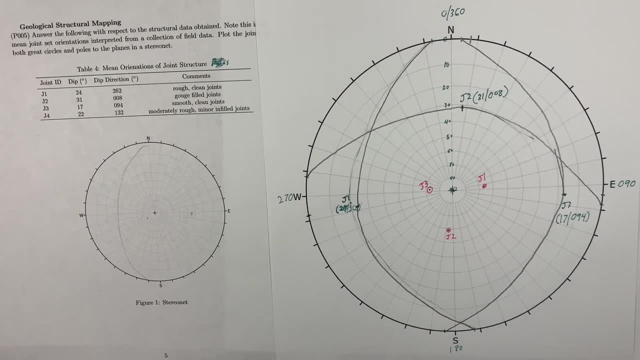 All right, so now we'll do the last one here. Okay, so J4 is in a direction of 132.. So 90, 100.. Okay, 100, 110, 120,, 132,, okay, And that has a dip of 22.. 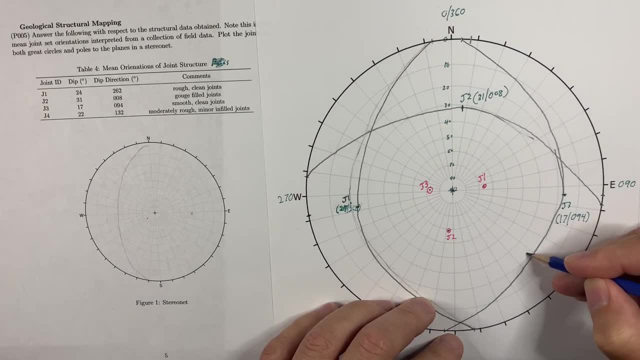 So 10, 22 is about here, okay, and I'm going to actually label this one right now. So that's J4, 22.. So that's J3, 22, and 132.. Okay, So let's draw the intersection with the outside so that we can draw our great circles. 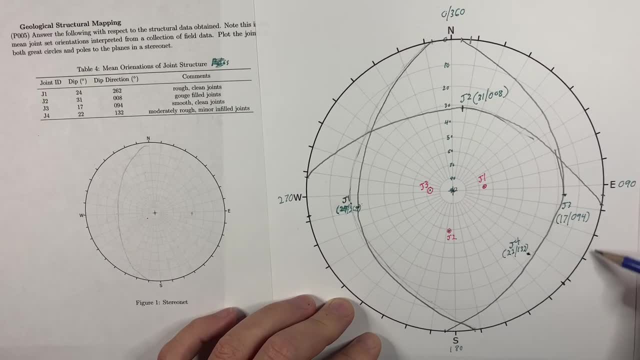 So we went past east by 10,, 20,, 30, 42 degrees. So let's do the same for north and south: 10, 20,, 30, 42.. 10, 20,, 30, 42.. 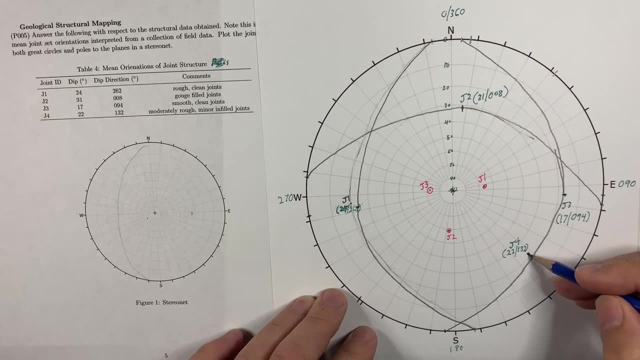 Okay, 9,, 9,, 11,, 12,, 13,, 14,, 15,, 16,, 17,, 18,, 19,, 20,, 21,, 22,, 23,, 24,, 25.. 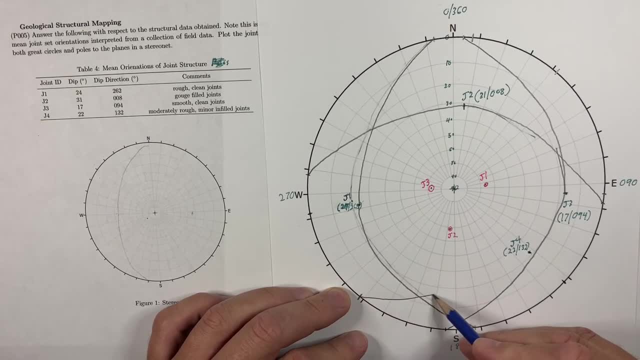 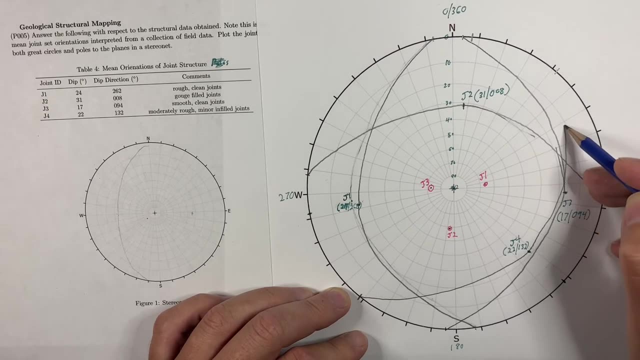 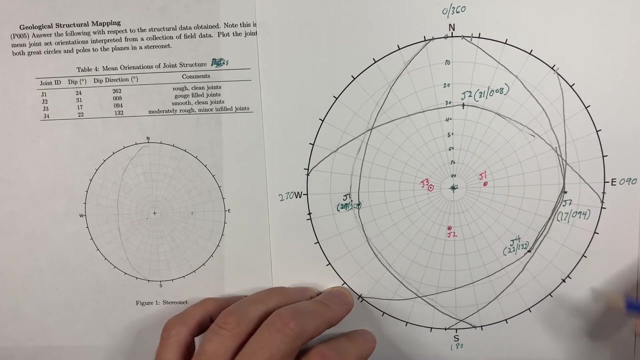 Okay, So now I'm going to do the last word of the day here. Okay, So I'm going to write this: Let me just draw a little bit of a circle for you, Okay. Okay, we want to draw the pole to that plane. Okay, so we're going to again line up the 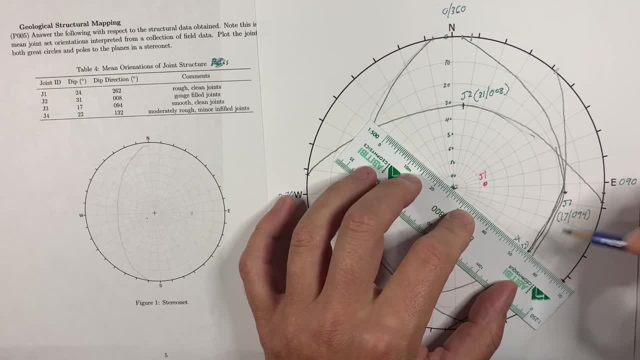 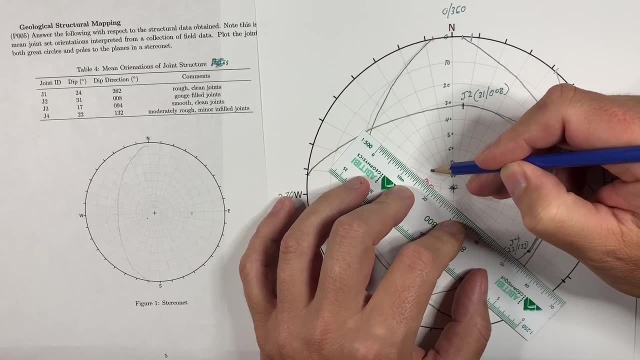 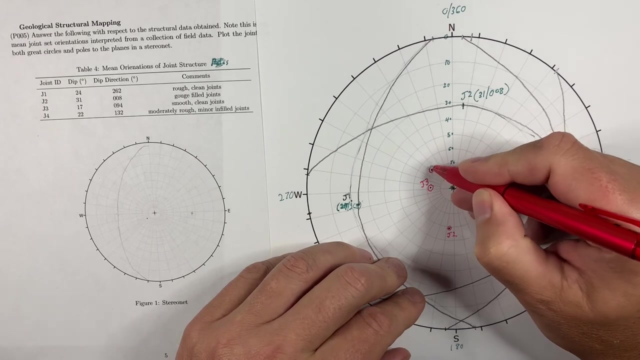 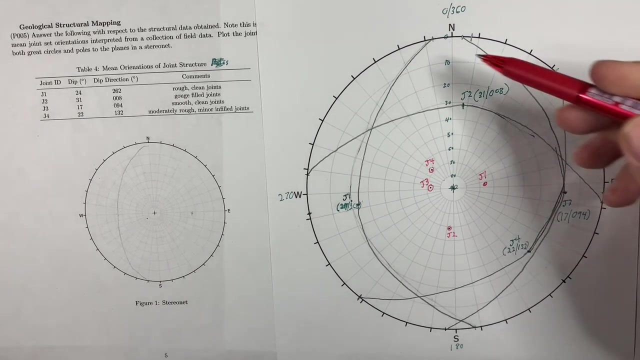 apex and go through the middle, and we want to go 22 degrees, 10, 22 degrees, Okay, and that is the pole of J4.. So again, just a reminder: the computer draws certainly much prettier structures and great circles than this, but really I want you to be able. 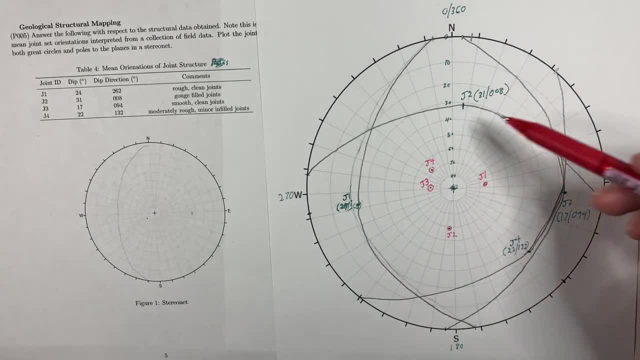 to understand how to plot them. Okay, so you get your great circles here, the apex points, and you get your apex points. Okay, so you get your apex points and you get your apex points. You know how to draw where they intersect the outside. Okay, and you know how to go. 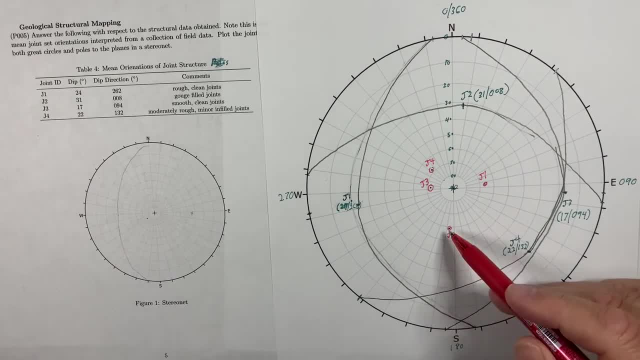 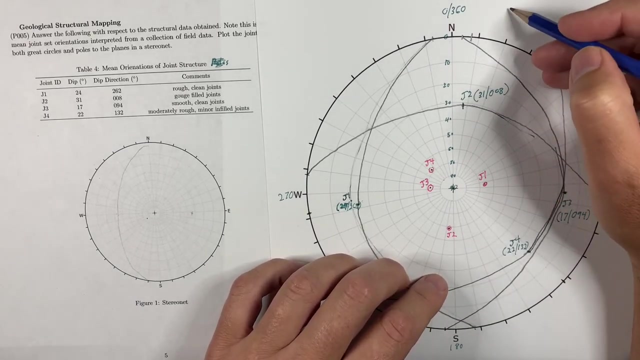 and get the pole. So you go 180 degrees around to get the direction of the pole and the dip is basically 90 degrees difference. So actually let me sort of show this as a calculation of the normal way to do it. So if you were going to look at the dip of the pole, 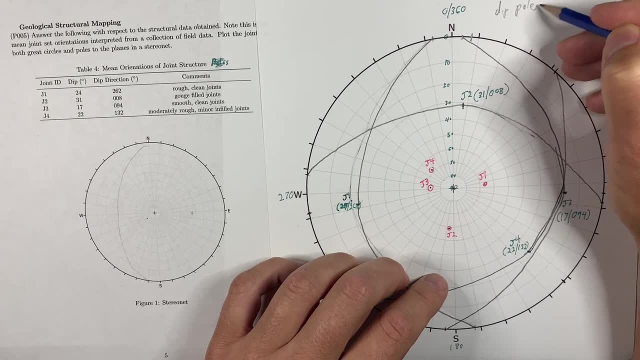 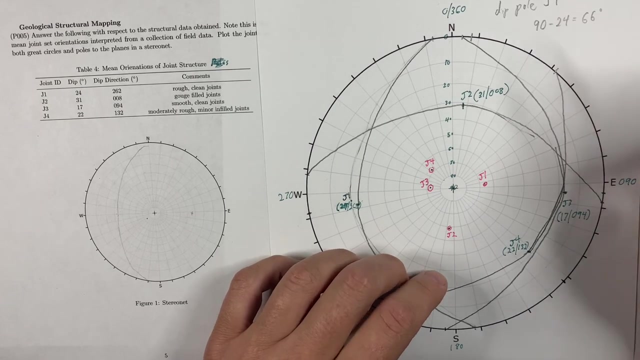 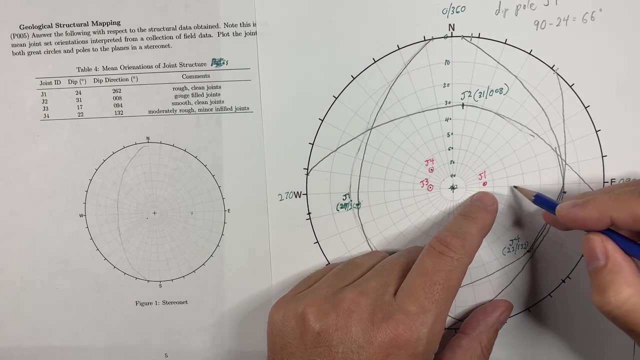 for, say J1 for instance: okay, 90 degrees minus 24 degrees is 66 degrees. Okay, so J1,, 10,, 20,, 30,, 40,, 50,, 60,, 6 degrees, right. 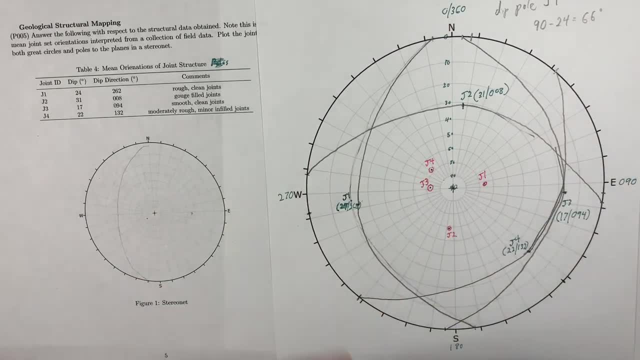 Or you could count 24 degrees. Okay, so J1,, 10,, 20,, 30,, 40,, 50,, 60,, 6 degrees. the force would be at 26 degrees from the surface of the process. to my theory,